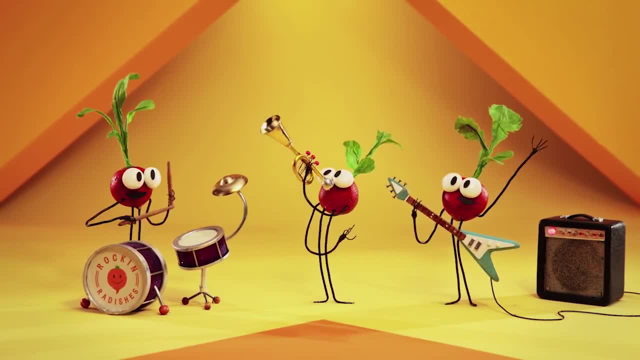 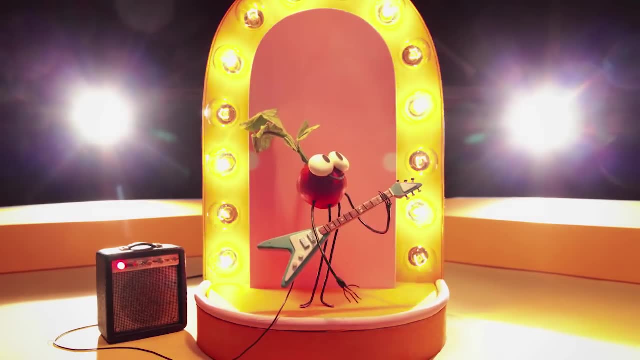 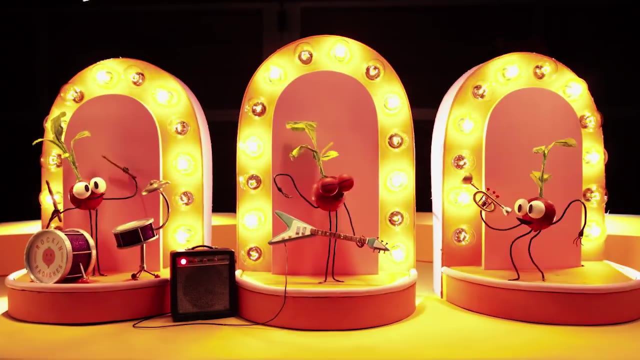 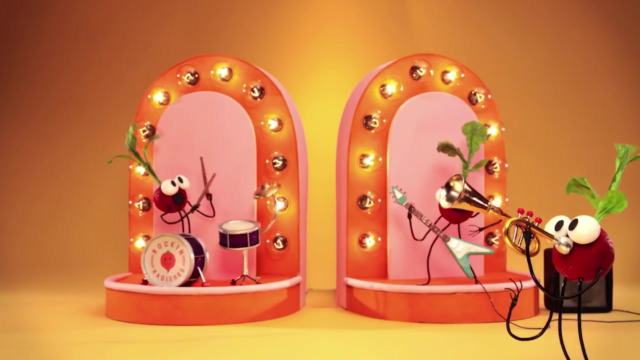 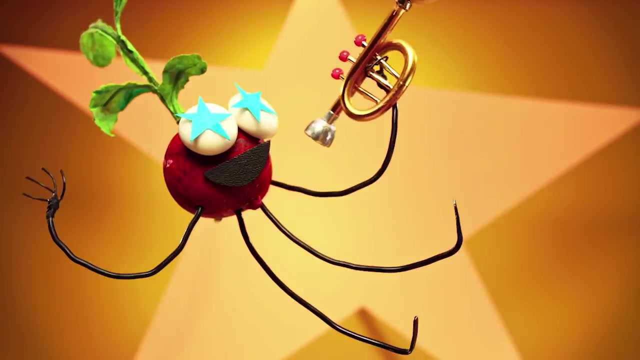 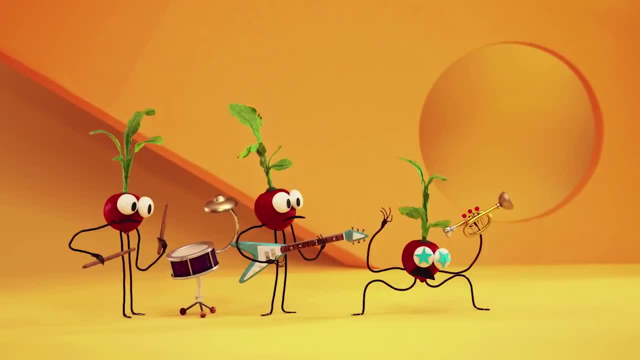 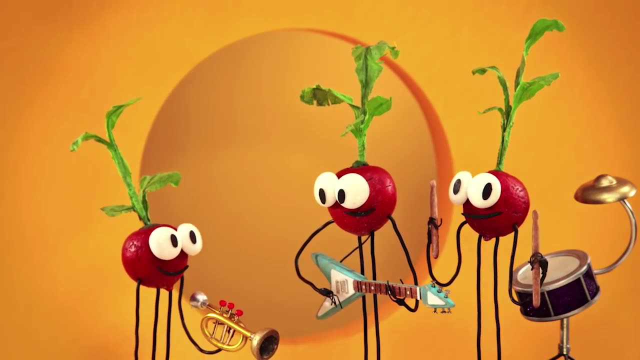 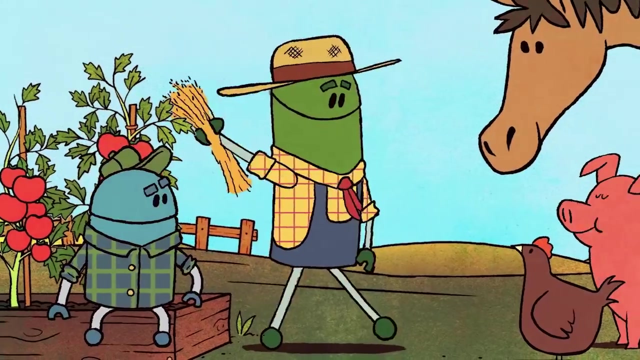 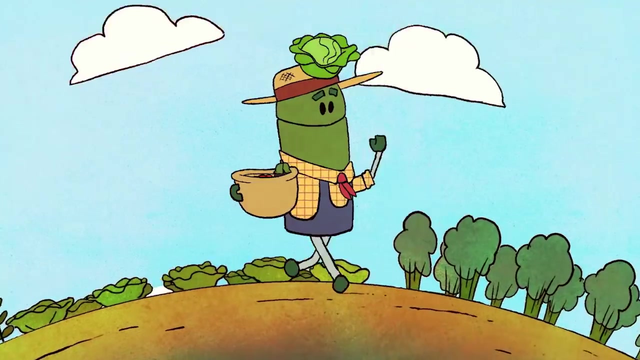 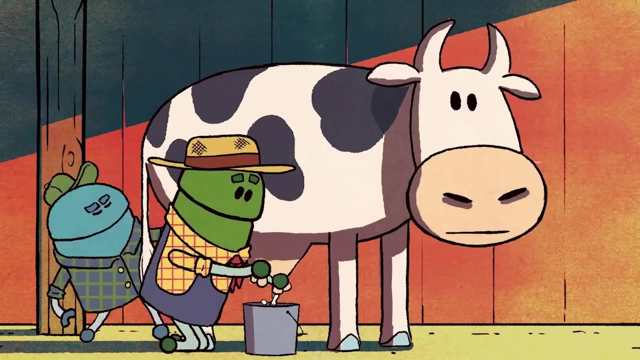 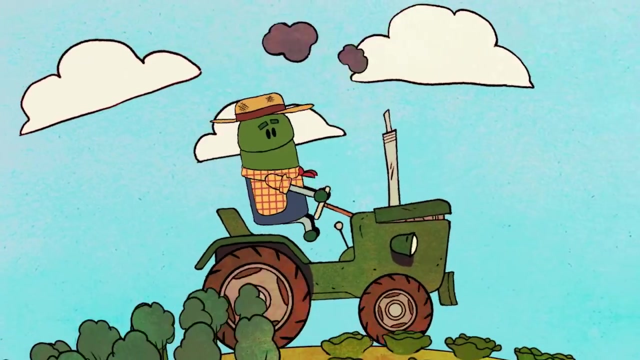 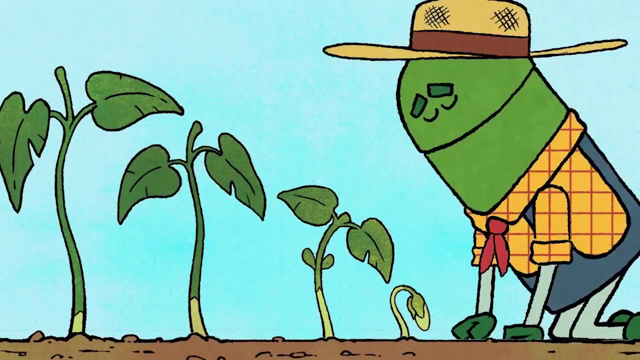 Radishes, Radishes, Radishes, Radishes. That'll soon be in the stores. That's how the farmer feeds the world: When cracking hens need chicken feed, When fields of hay need mowing, When beans and greens need watering To keep them strong and growing. 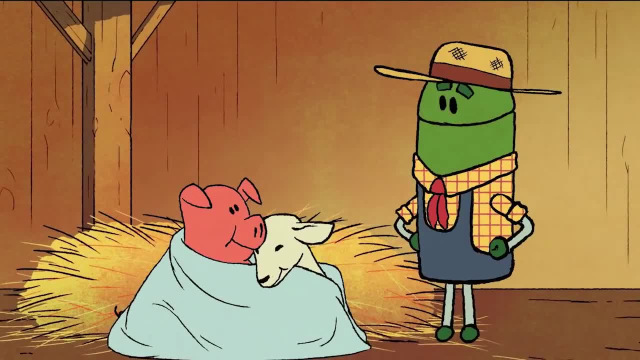 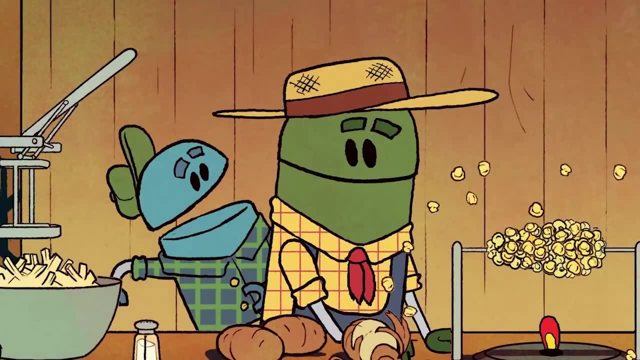 When pigs and lambs need extra care Cause winter winds are blowing, The farmer is always on the job. Whenever we eat french fries Or delicious corn that pops From scrambled eggs to chicken legs, To burgers, steaks and chops, They all come from the friendly farmers, Animals and crops. 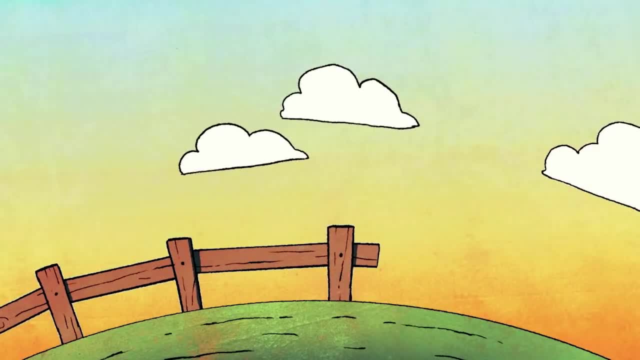 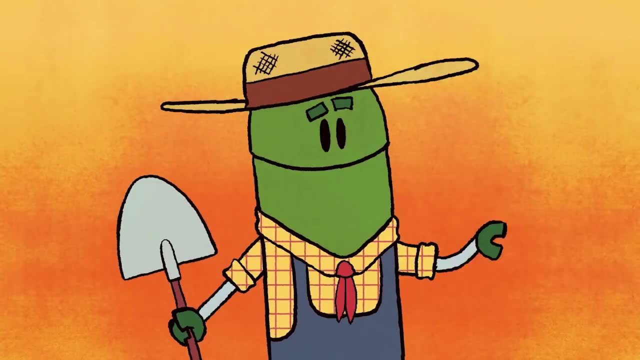 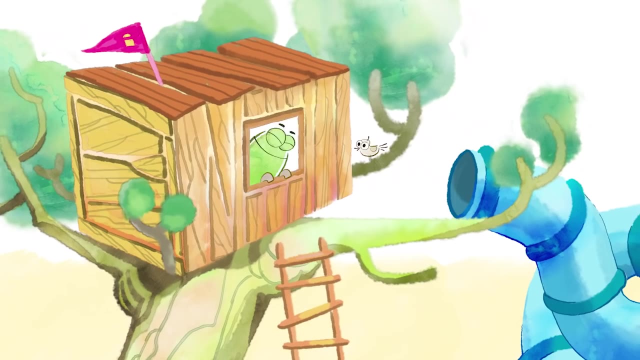 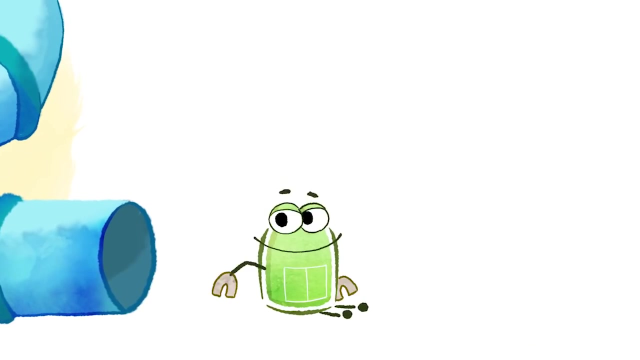 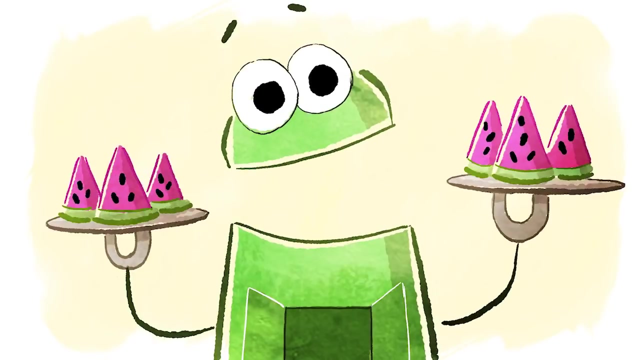 That's how the farmer feeds the world. That's how the farmer feeds the world, Fulfilling all our grocery needs With just some water, dirt and seeds. That's how the farmer feeds the world. Stuff, our yummy treats can make you happy, And you may wanna run around, giggle, play or be a clown. 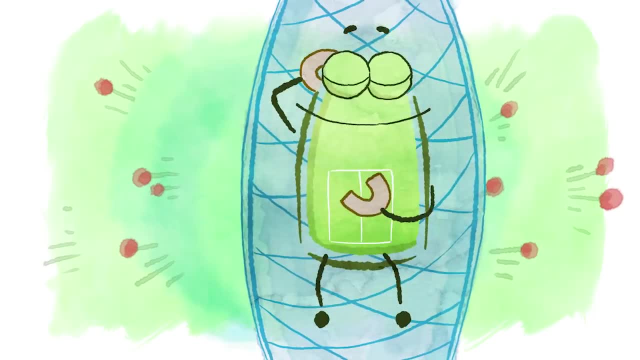 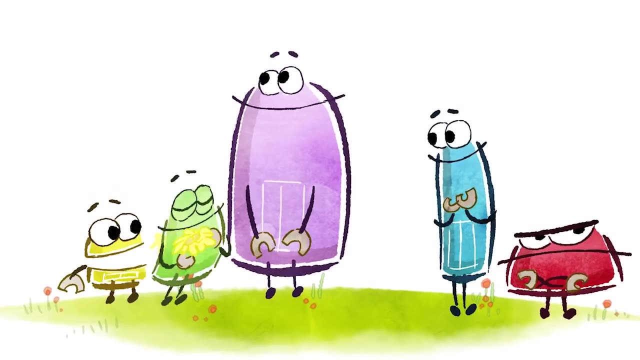 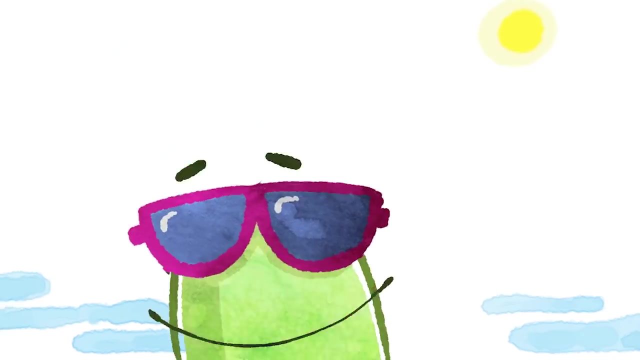 When you're happy, When you feel good inside, all warm and satisfied, You know you're happy, happy, happy When you can spread around all of the joy you've found. When you are happy, happy, happy. Happiness can come in waves Made of all the smiles you gave. 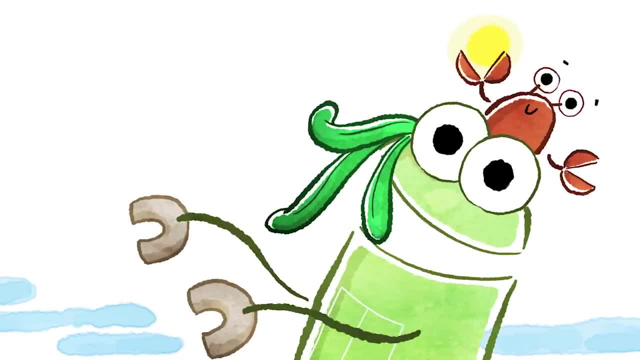 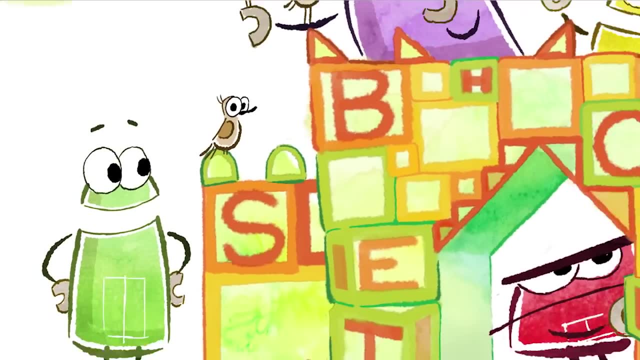 Things may not go your way, but everything is still okay When you're happy And you will wanna jump for joy. Even show your favorite toys when you're happy, Up down front and behind. Brush them all around Till they sparkle and shine, Cause cavities are meanies. 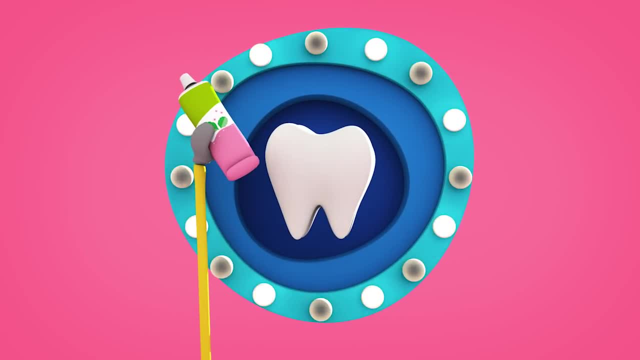 And meanies don't belong in your mouth. So everybody do the Ch-ch-ch-ch-ch-ch. Like you're gonna start, ya Go. Ch-ch-ch-ch-ch-ch-ch, Ch-ch-ch-ch-ch-ch, Ch-ch-ch-ch-ch-ch, Ch-ch-ch-ch-ch-ch. 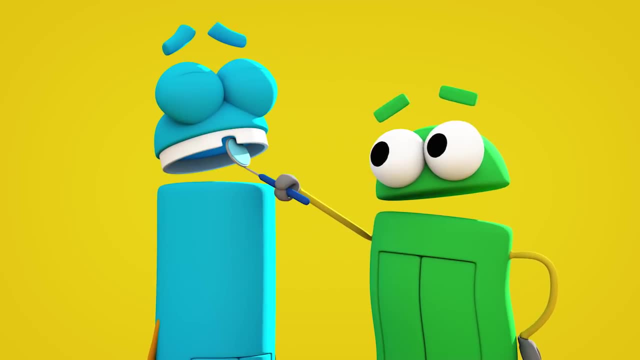 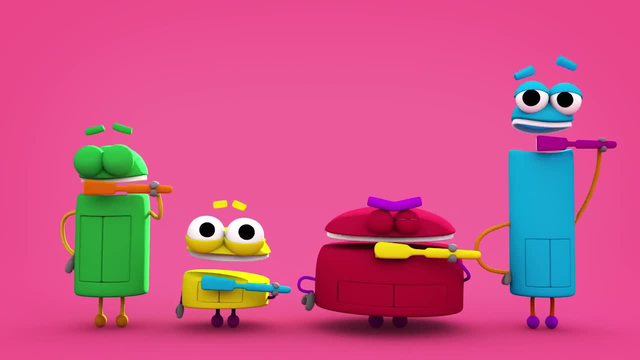 Ch-ch-ch-ch-ch-ch. Like you're gonna start, ya Go Ch-ch-ch-ch-ch-ch-ch, Ch-ch-ch-ch-ch-ch, Ch-ch-ch-ch-ch-ch, Ch-ch-ch-ch-ch-ch. If ya like to nibble, not bite, Munch and punch. If you like chewing and chomping. 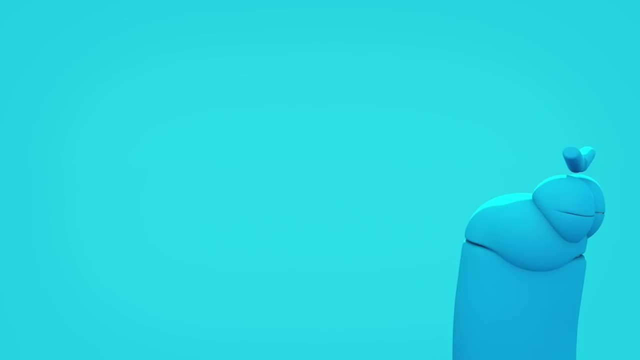 Then chow and have lunch. Then don't brush Like you're in a rush, Scrub em' every which way. So everyone do the Ch-ch-ch-ch-ch-ch-ch. Now all together do the Venom-mm-mmm- GoPro, Don't be thumbnail. So everybody do the. 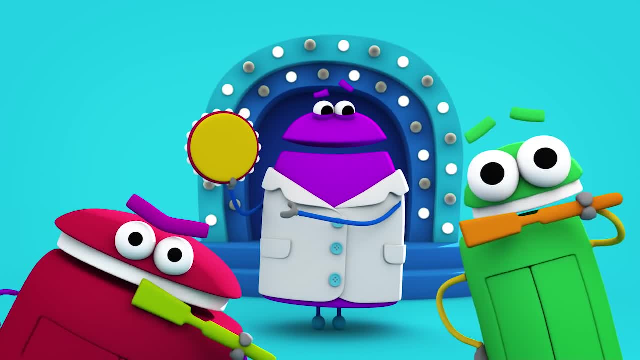 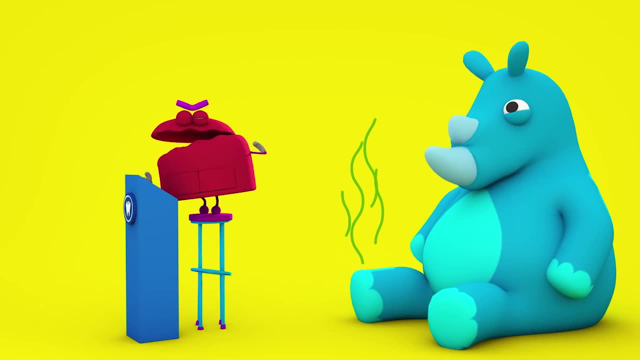 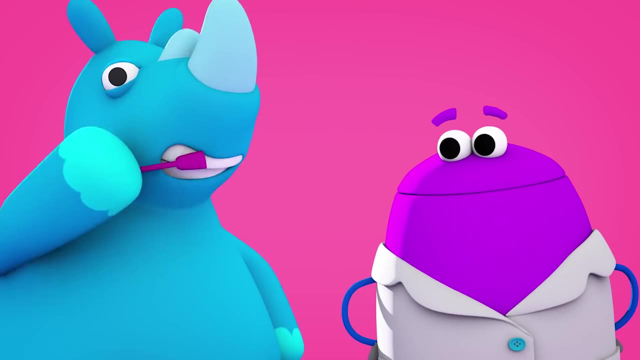 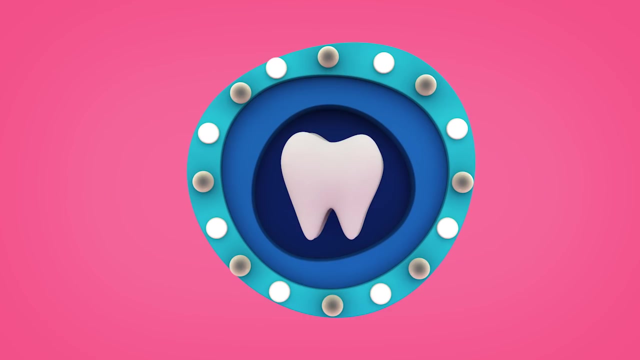 Now, all together, do the, And when you open your mouth to speak, You don't want your breath smelling like rhinoceros feet, So you better brush up on your brush. Everybody do the Like you're Dennis Dodger. Come on, people do the. Go, brush your teeth. 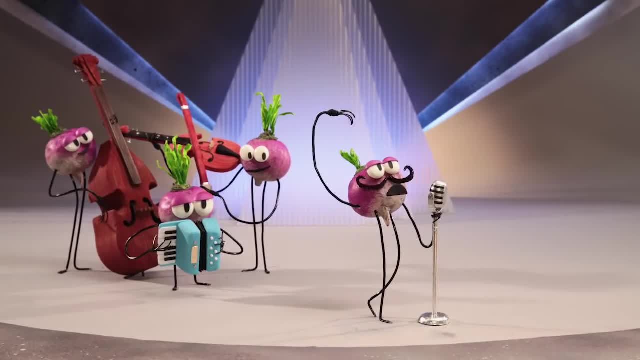 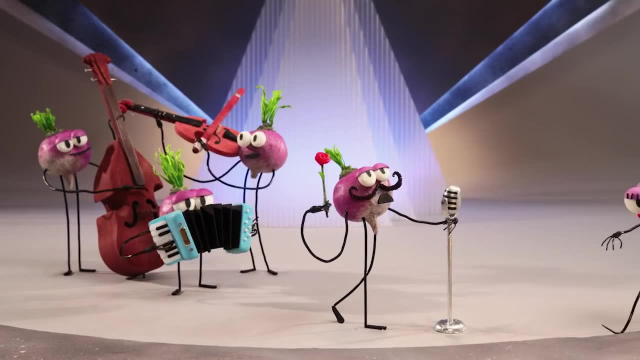 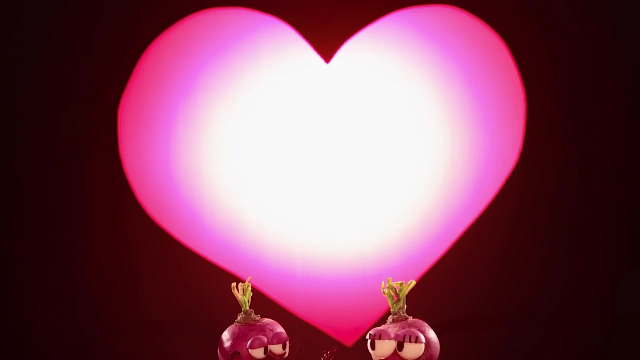 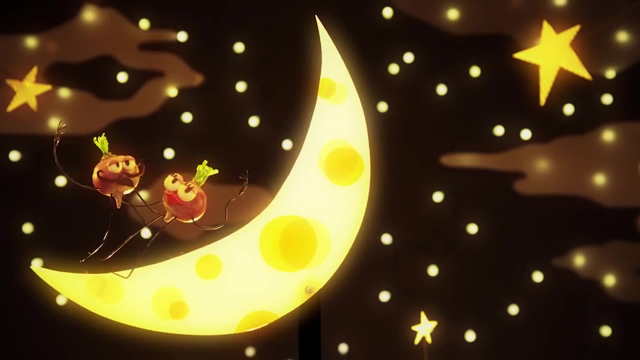 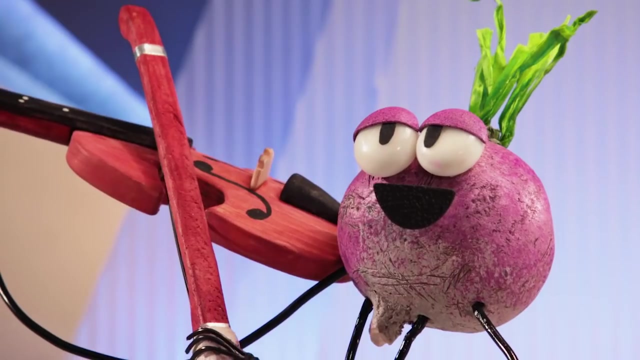 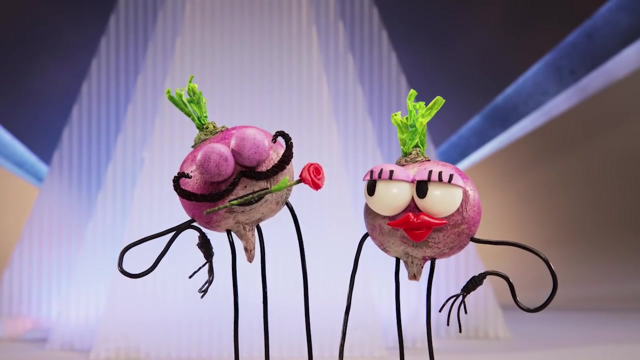 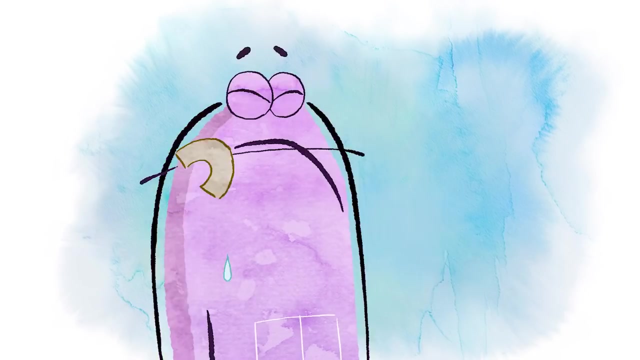 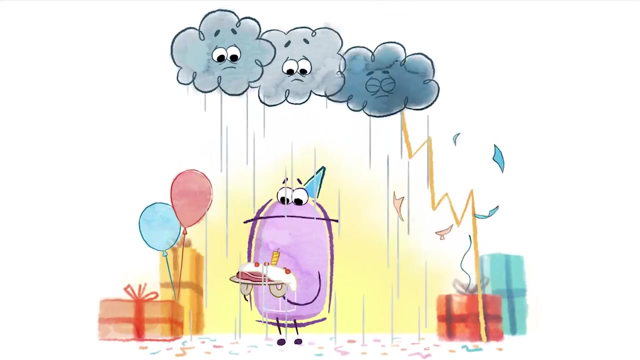 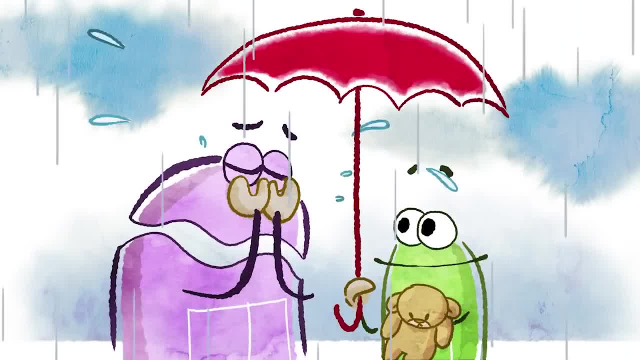 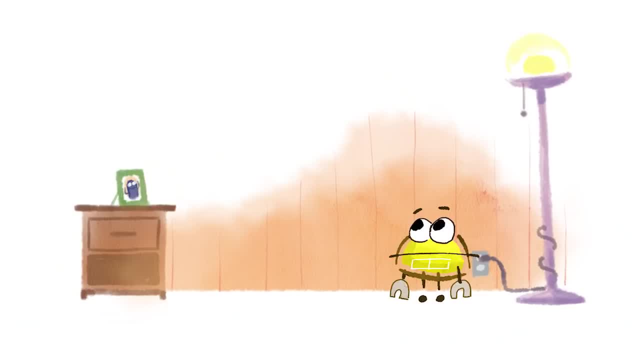 Just up and hopping to you. So don't despair. find someone who cares. A cuddle with Teddy will do When you feel yucky inside of you. Are you going to hide And these feelings stick to you? Tell someone why you have tears in your eyes And ask for a hug or two. 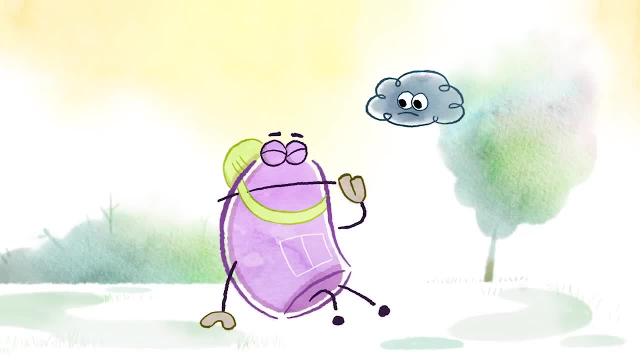 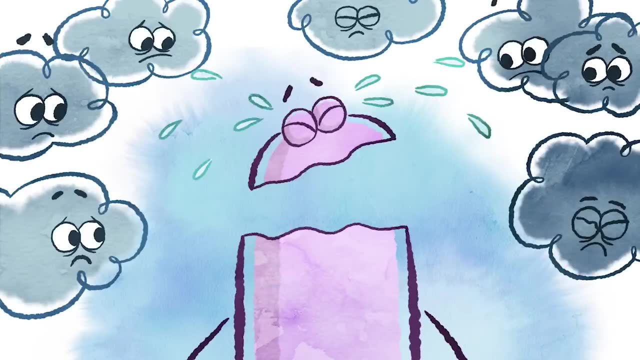 It's not so bad to feel a little sad Sometimes, what you gotta do. When you need to cry, Let the teardrops fly. When you need to sneeze, Go achoo and have a little pout, But let it all out. It's always the best thing to do. 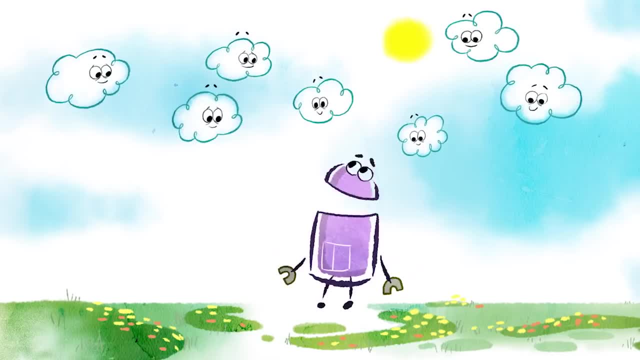 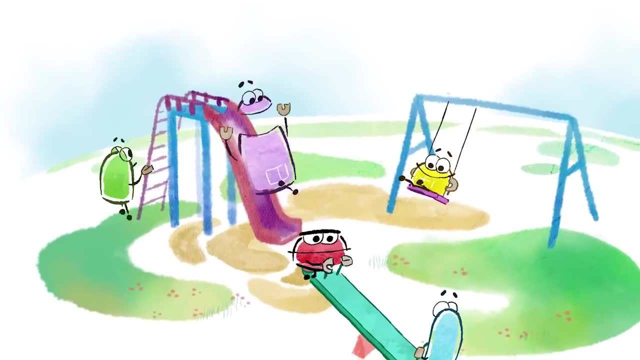 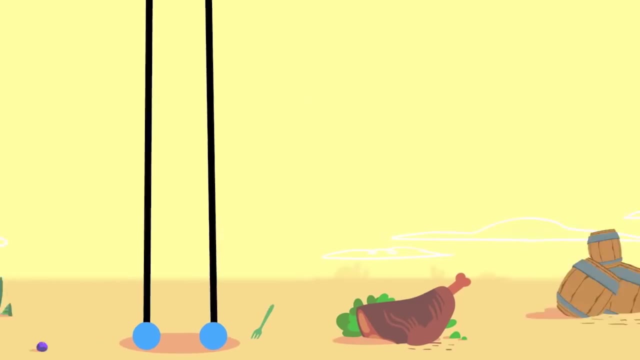 Just have a good cry and say goodbye To feeling sad and blue. Just have a good cry and say goodbye To feeling sad and blue When fresh food is what you need To be strong and healthy as you're growing And your tummy is like a gas tank. 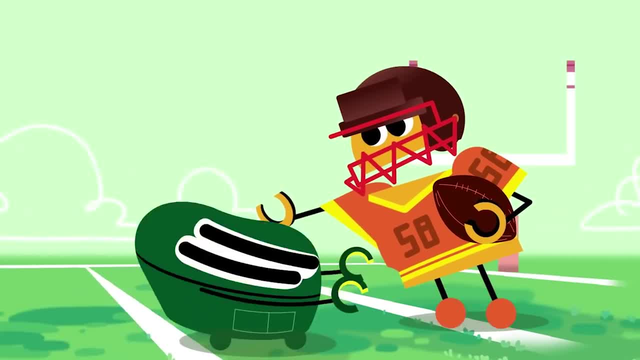 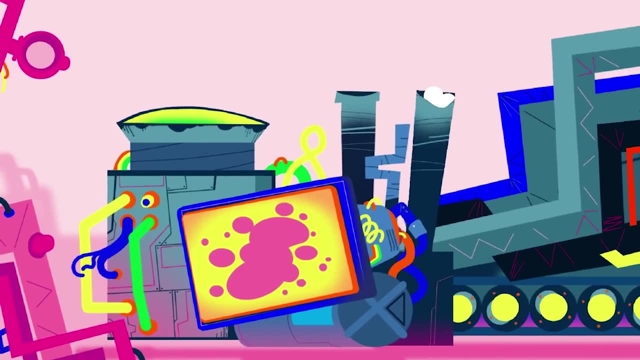 That you fill up when you want to get going. Then you can play, you can run, You can have lots of fun And dance all around till the day is done. Your stomach is like a factory Turning food into energy. What you eat is yummy from your mouth. 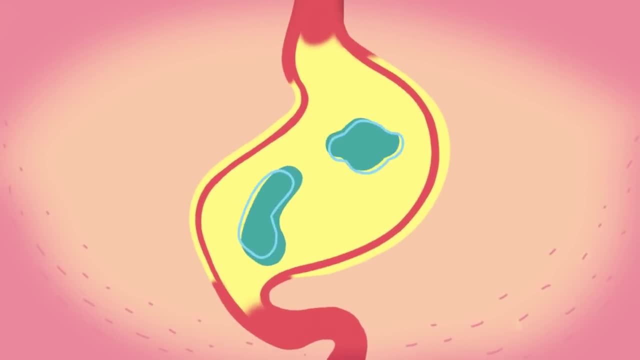 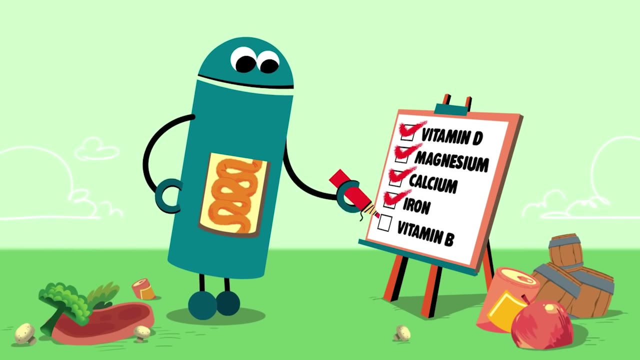 To your tummy as it travels down your esophagus, Where it hangs out in your stomach Mixing up so it can digest. Then your food passes through your small body To your small intestine, Where your body gets everything it needs To build your muscles, Make you grow. 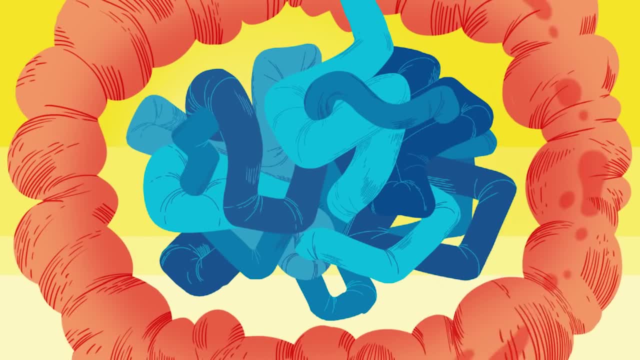 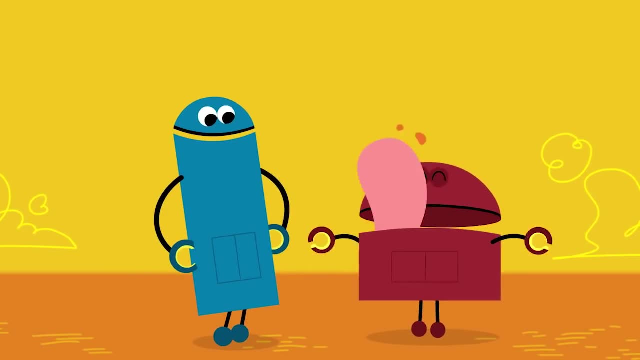 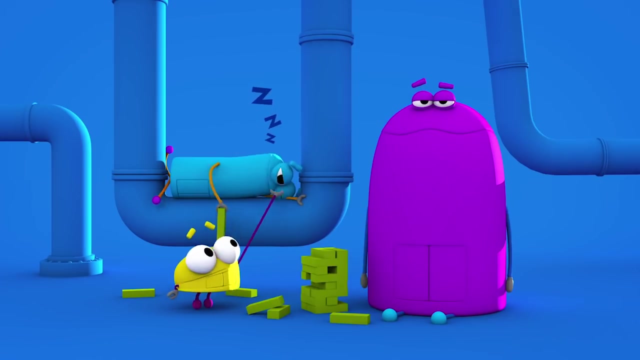 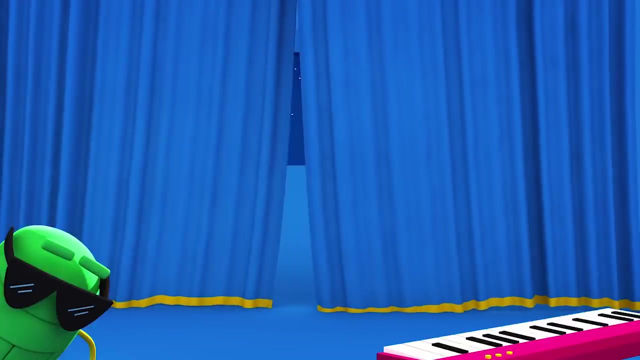 Give you lots of energy, Then what's not used just passes through. Some people call it number two. Your digestive system is your factory Turning food into energy. It's time to catch some Z's And recharge your batteries. So come on, come on, The curtain's drawn. 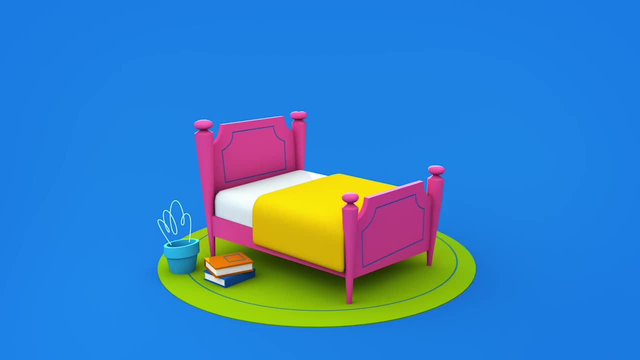 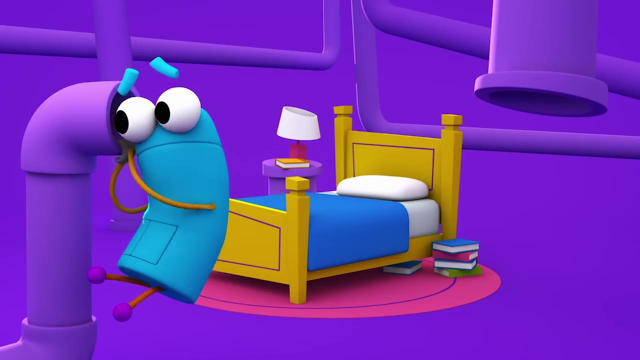 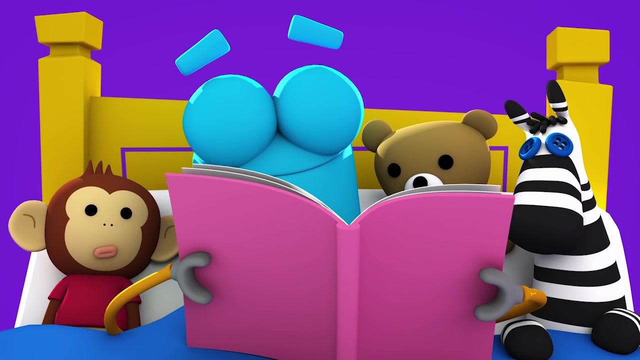 So begin your all-night snooze-a-thon. It's time to get in bed. You can dream of soaring through the air. It's time to get in bed, Snuggle up to your favorite teddy bear Or chip or whatever, Even if you feel wide awake. 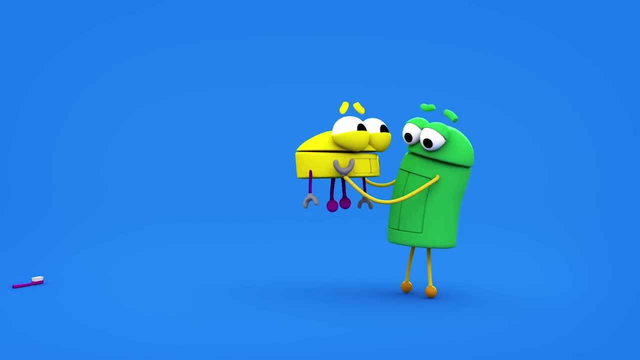 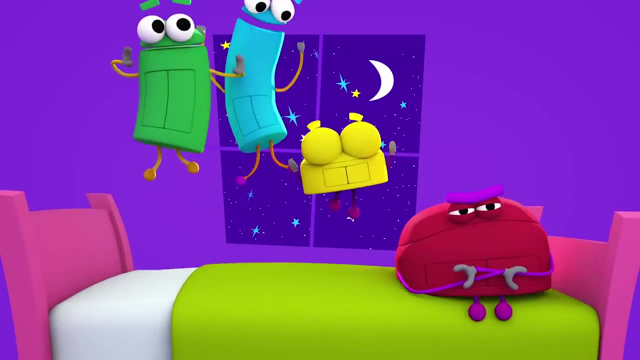 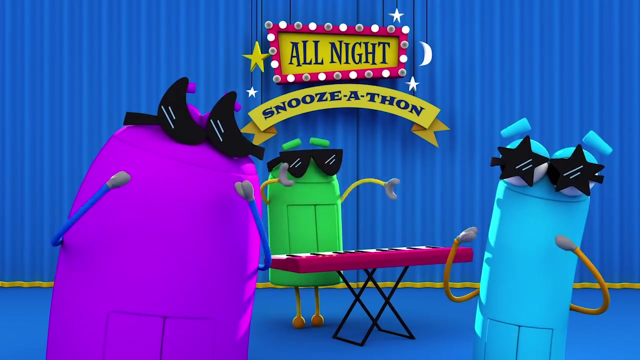 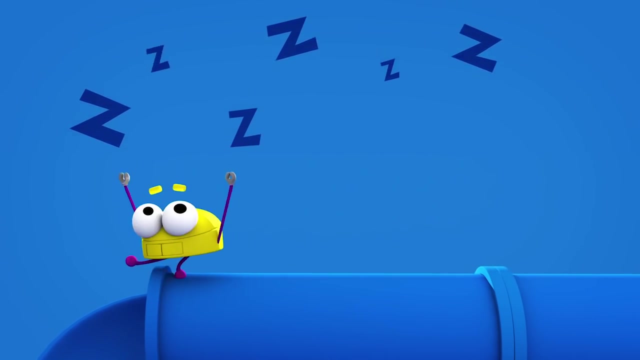 You still need sleep, for heaven's sake, And staying up late will seal your fate To be a total cranky pants. Whoever said you snooze, you lose, Was clearly quite confused, Because it's time to get in bed. Sleepyheads report for duty: It's time to get in bed. 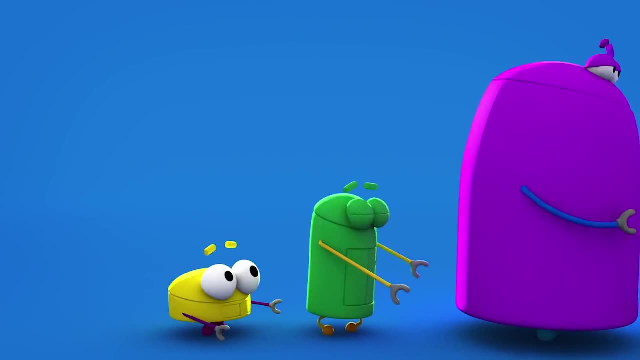 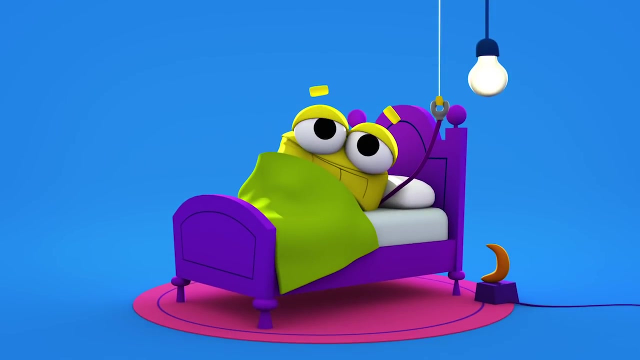 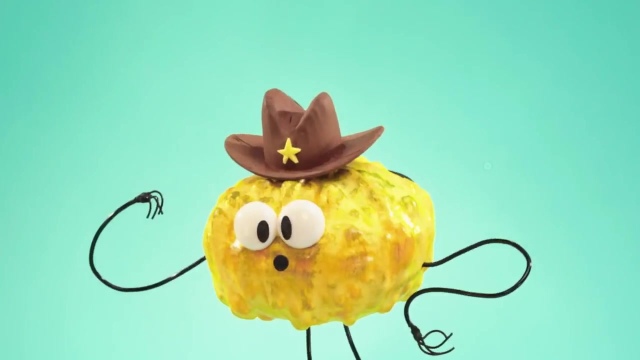 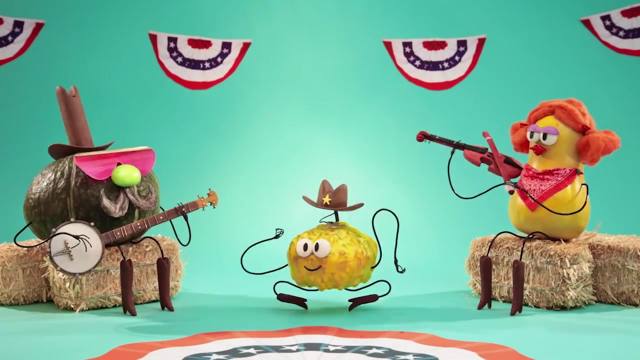 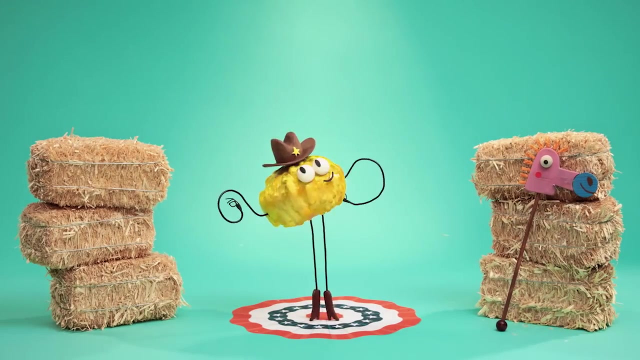 Everybody, let's get snoozy tonight. The world's turning off its lights, And so should you. And because it is? Because there are No more, No younger And no longer Shortages, No longer, No one, No more Zero, No one More Overturn And then destroy Every other learned human being. 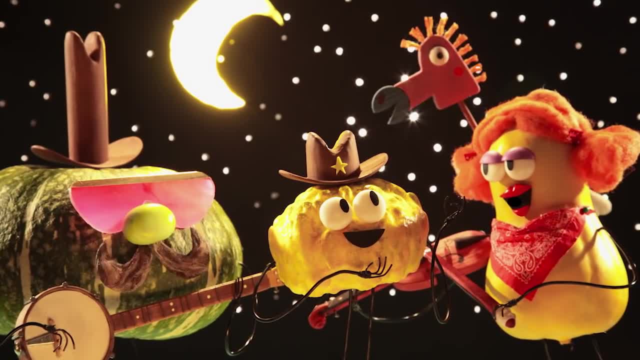 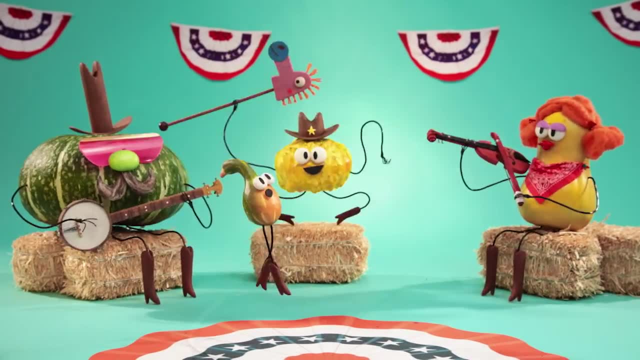 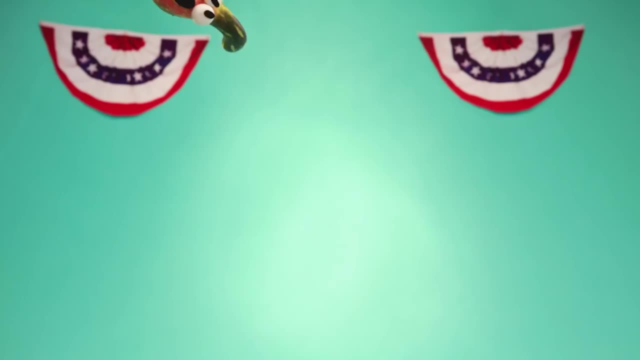 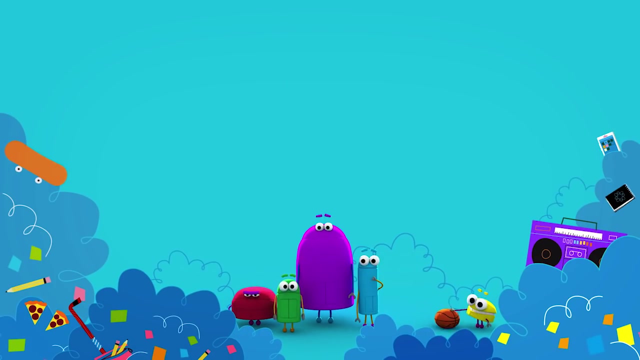 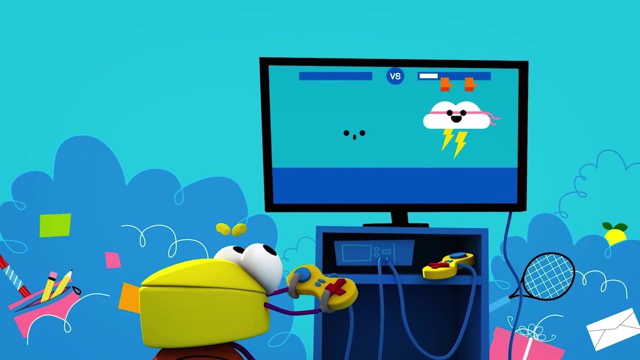 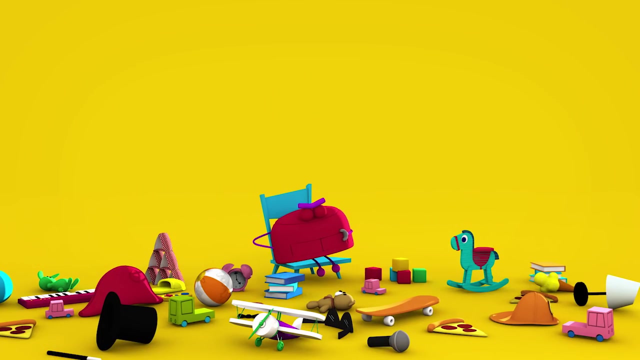 Do whatever it takes. According To A Modal Life, No offense, but this place is a giant mess. In fact, it looks kinda like a hurricane Pick a fight with a tornado. A disaster top to bottom. So put these toys back where you got them, Because rooms don't clean themselves. 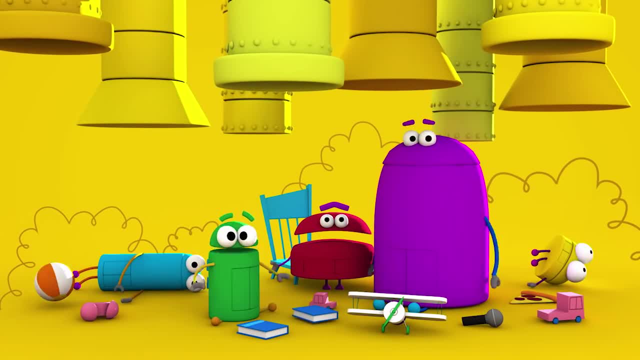 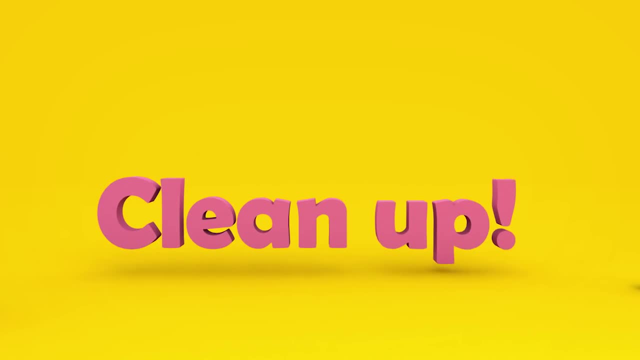 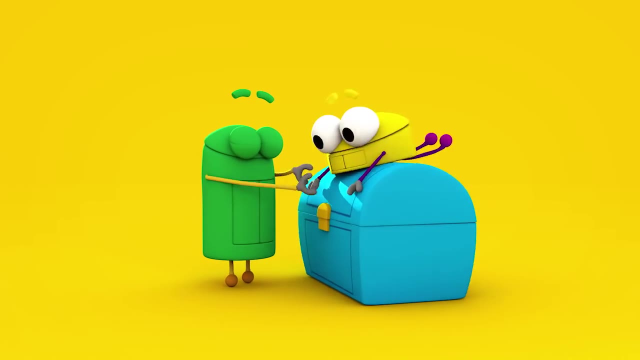 Though if they did well, that'd be awesome. But those haven't been designed, So now it's clean-up time. Go clean up, clean up. Come on, it's clean-up time. Some things go in boxes. Some things of yours belong in drawers. Some things go in closets. 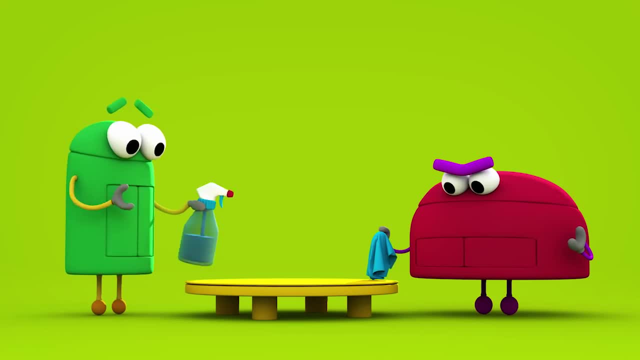 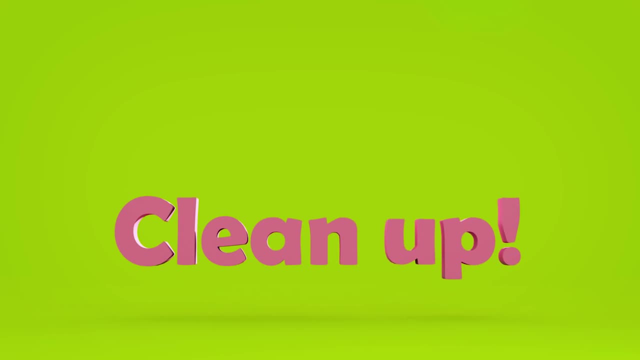 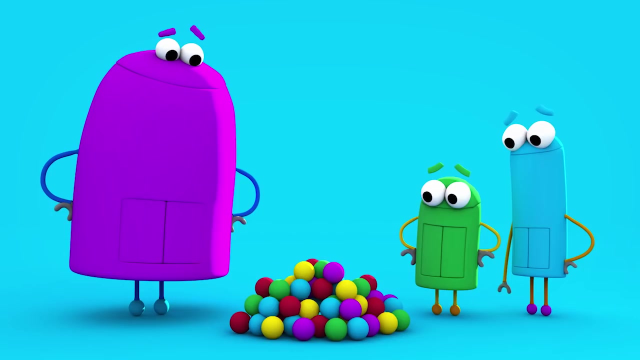 So pick those things up Off the floor, Because the bottom line Is that it's clean-up time. So clean up, clean up. Come on, it's clean-up time. It's more fun to make the mess than clean it. Nonetheless, I mean it, It's clean-up time. 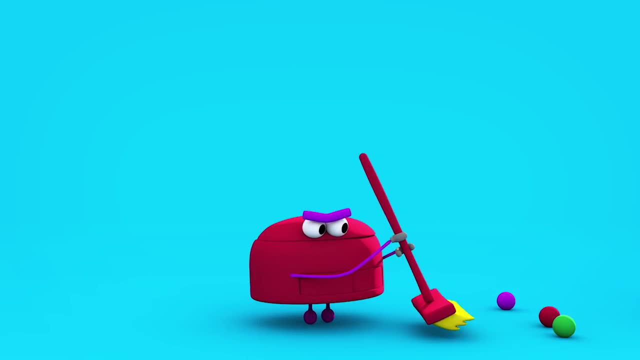 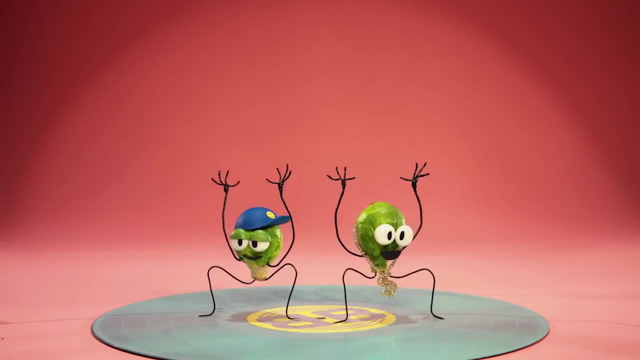 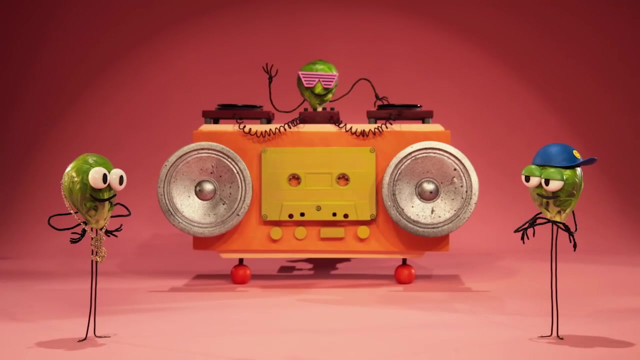 It's clean-up time. Go Brucie. It's clean-up time. Go Brucie, Do it. Go Brucie. It's clean-up time, Go Brucie, Go Brucie In the roll OSUE Yeah. 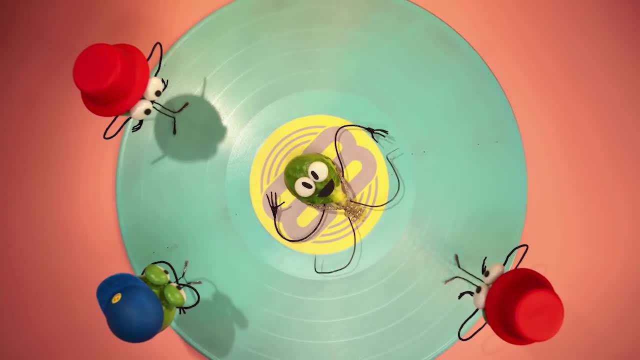 Go Brucie, It's clean-up time. Yeah, yeah, yeah, go, Yeah, Nate. Yeah, yeah, I'd be fine. Oh yeah, Chicken, chicken, All 4D. get down Brucie, Go, get down Brucie.